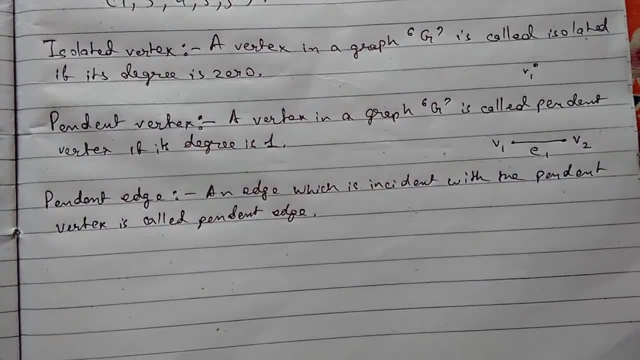 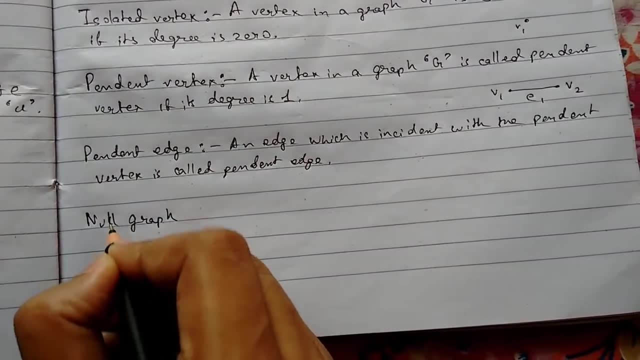 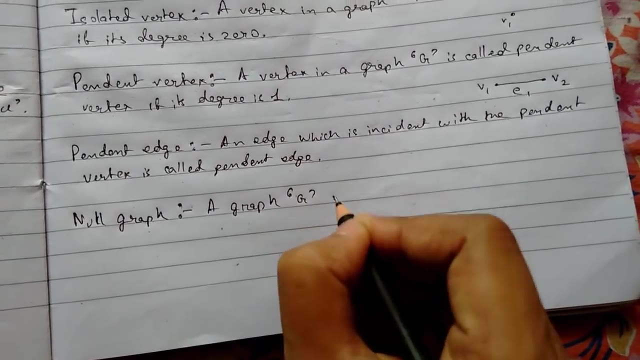 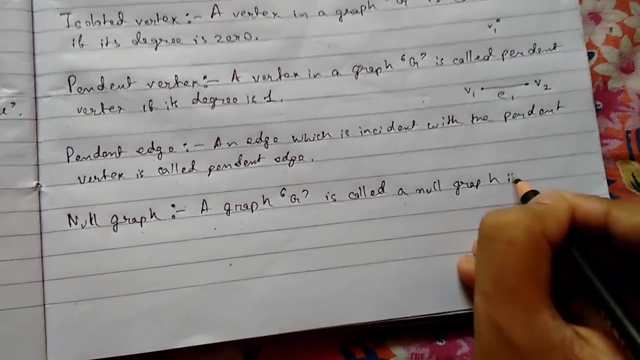 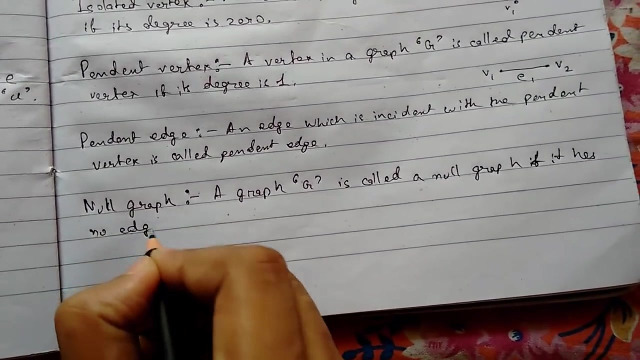 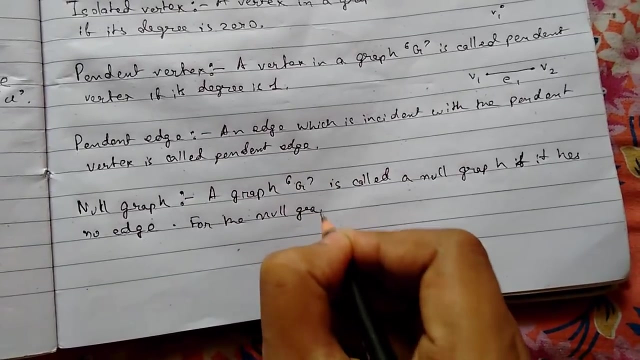 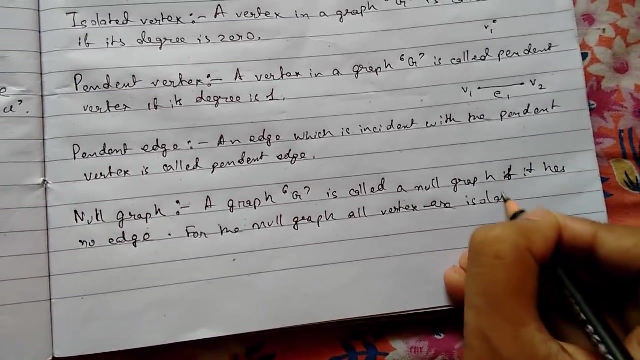 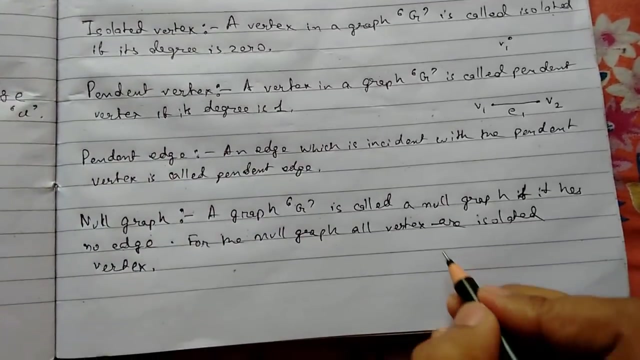 so it will be known as the pendent edge. now let us start null graph. so a graph G is called a null graph if, if it has no edge for the null graph, all vertex are isolated vertex. so basically, to have a null graph, you should have an isolated vertex. so v1, v2, v3, so 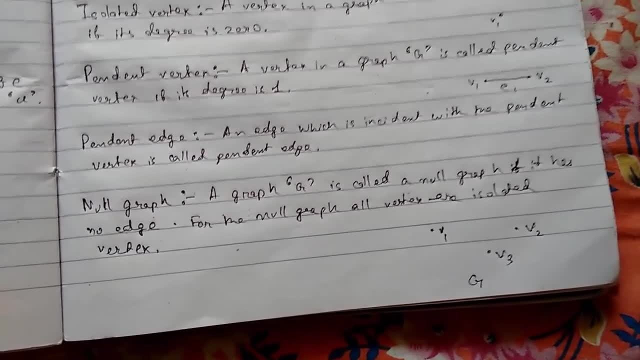 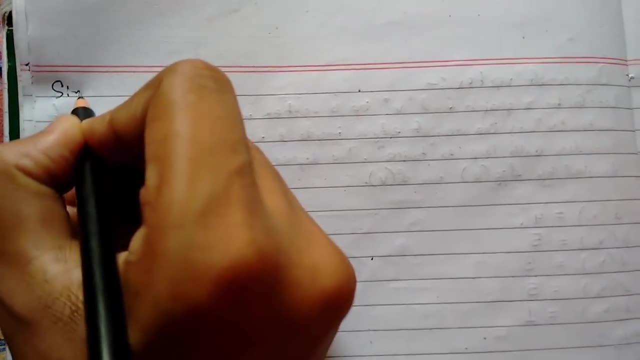 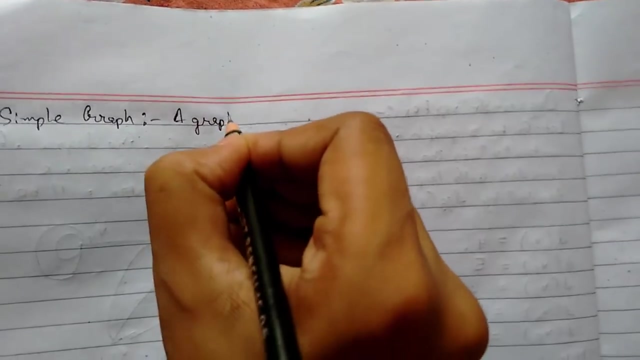 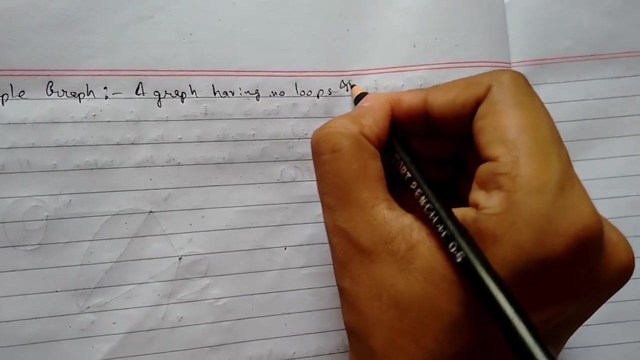 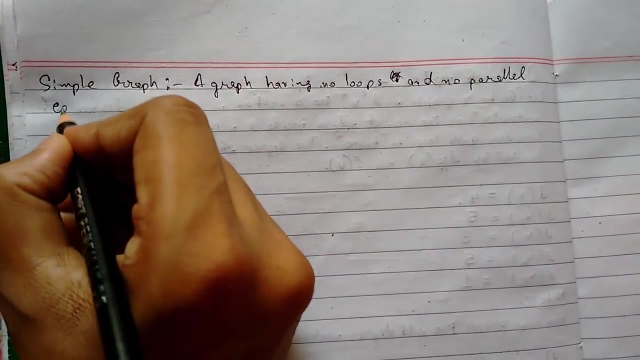 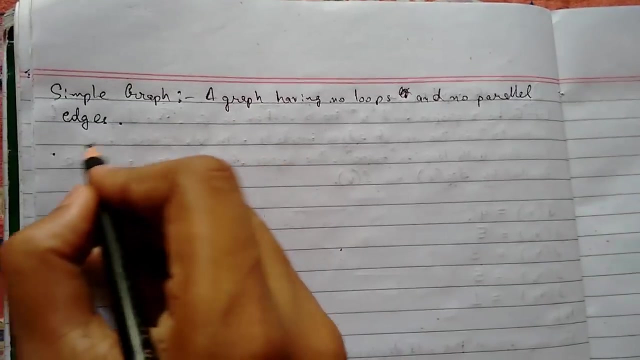 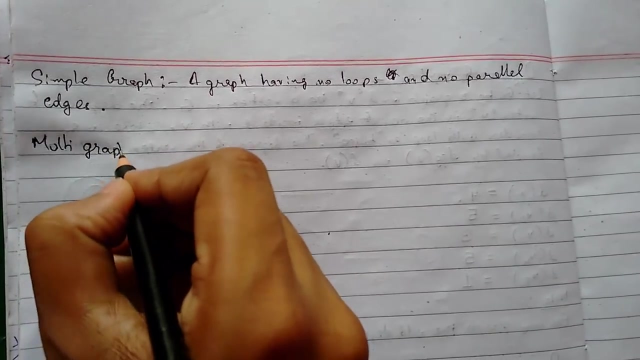 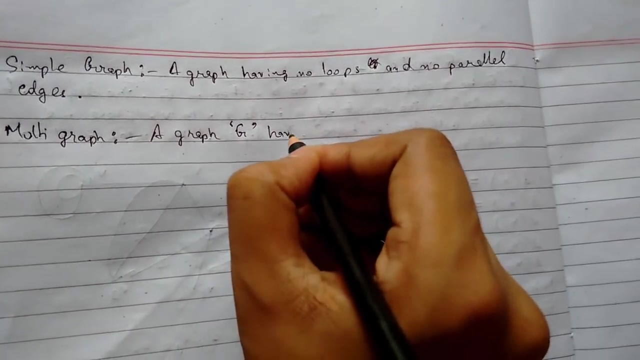 this is all a graph G which has three vertices. so this is a null graph. now we'll see simple graph. so a graph having no loops or self loops and no parallel edges. no parallel edges is called a simple, simple graph. so I will explain this by this multi graph. so a graph G having no self loops. 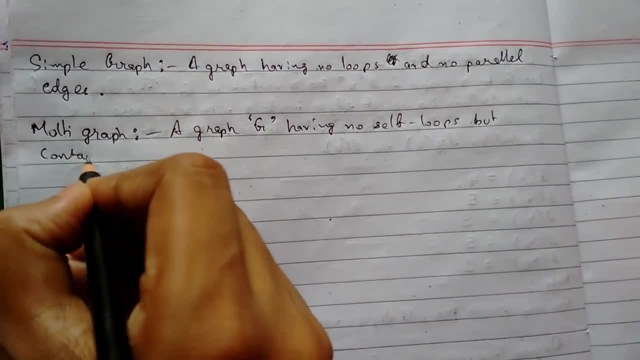 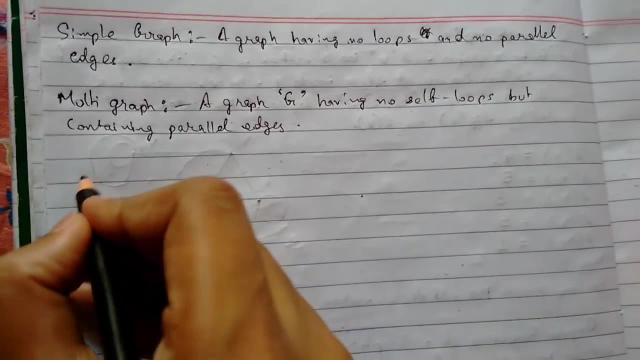 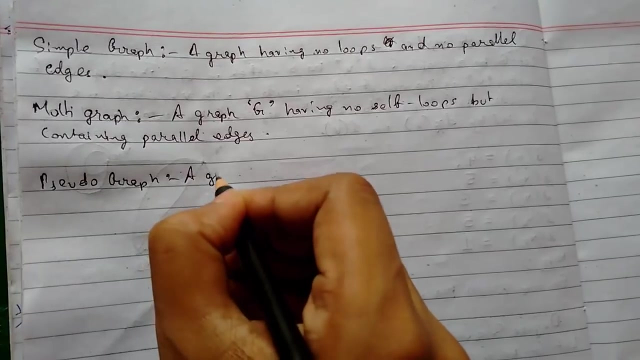 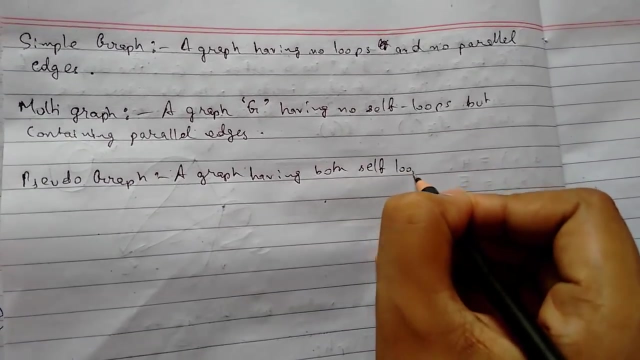 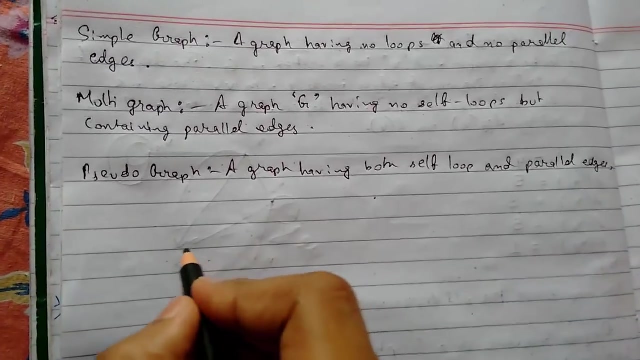 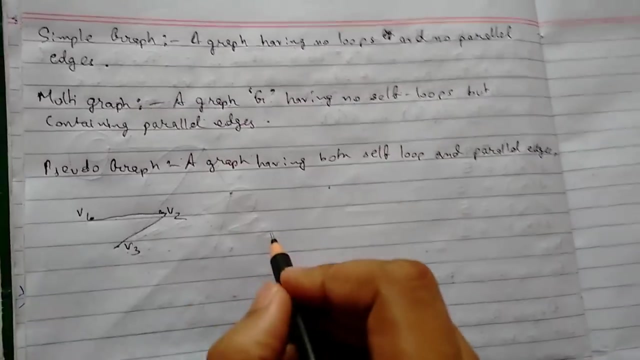 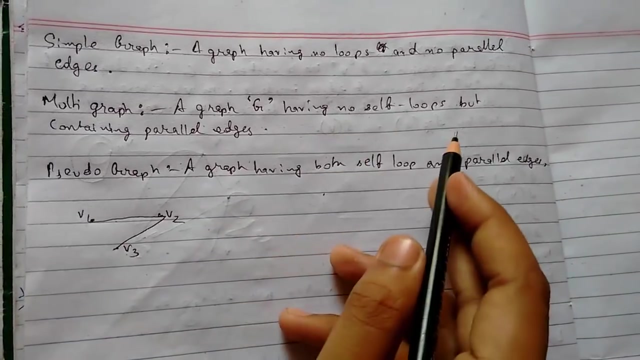 but containing parallel edges. now, pseudo graph, a graph having both self loops and parallel edges. so so so for simple graph, it should be something like this: v1, v2, v3, like this for multi graph is: should have, is not have any yourself for parallel edges, for multi graph having no self. 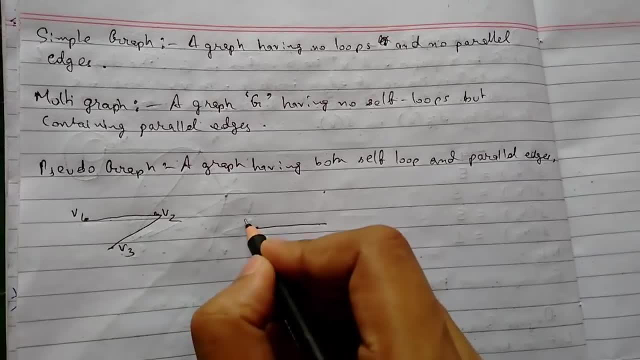 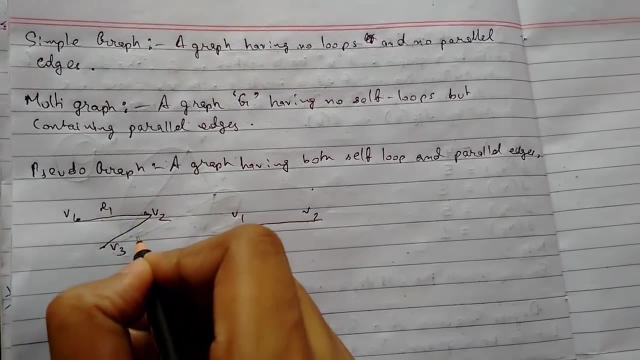 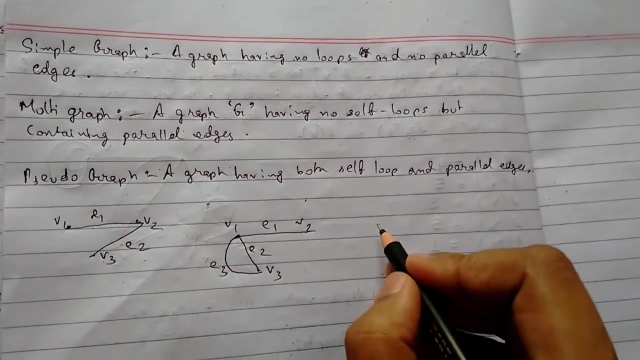 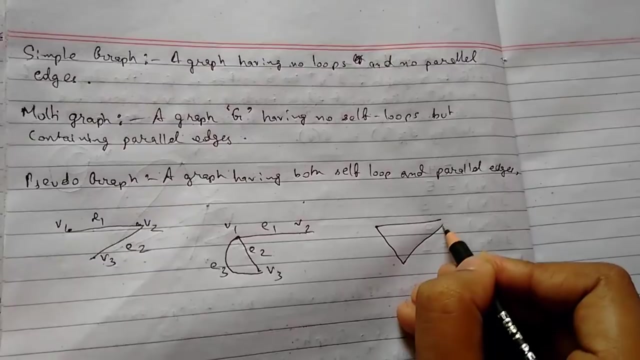 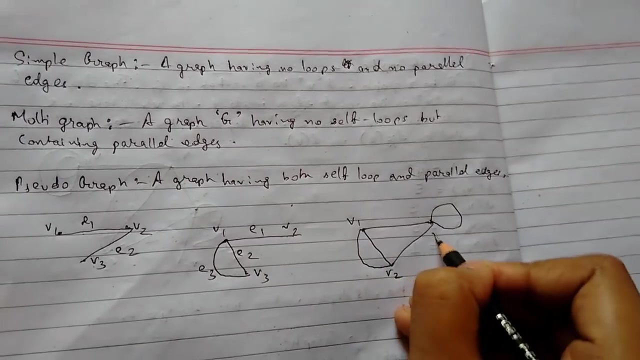 loops but containing parallel edges. so something like this: v1, v2, v3. so this is e1, e2. here it will be. here we see that there are two parallel edges and for pseudo graph it should have both: V1, V2, V3, E1, E2, E3, E4, E5. 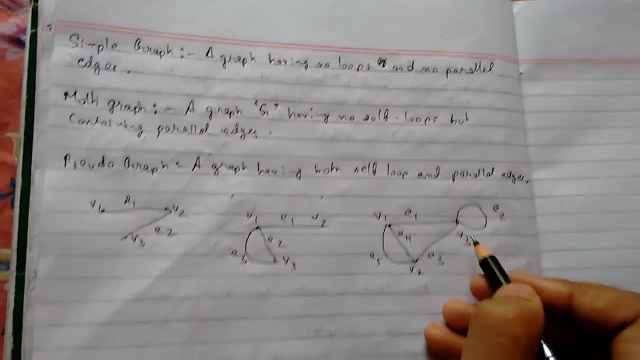 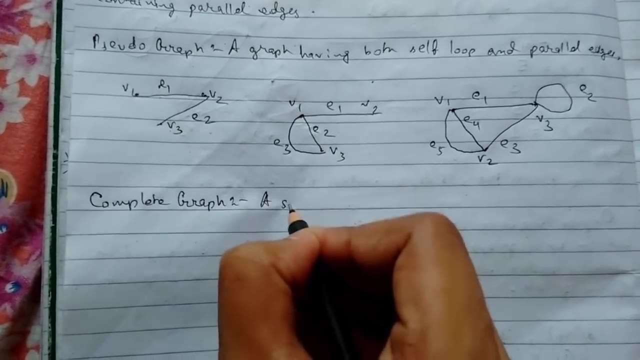 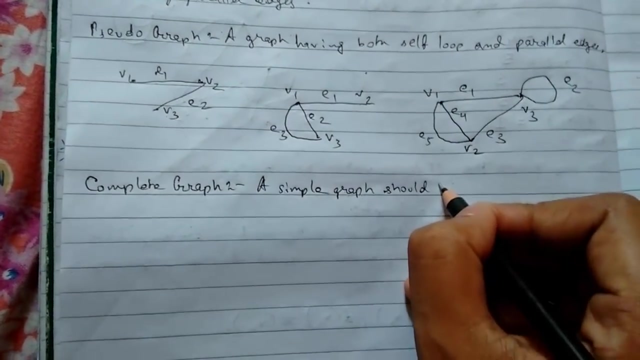 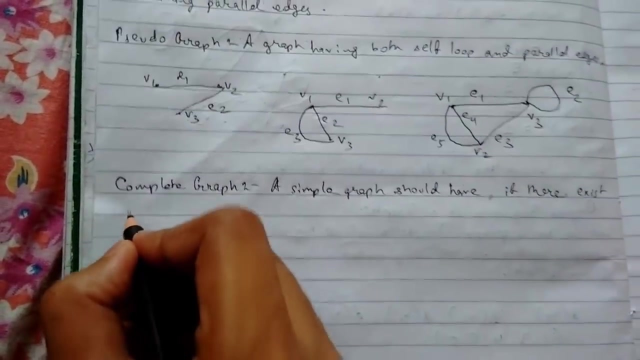 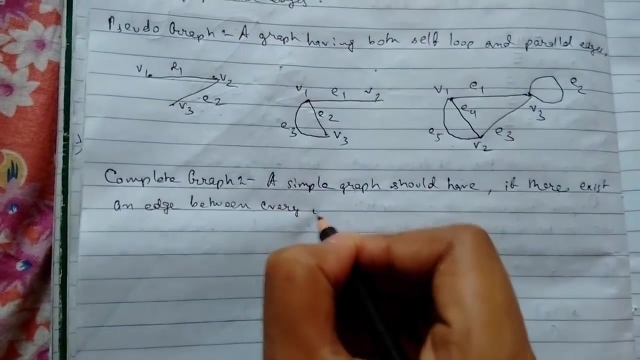 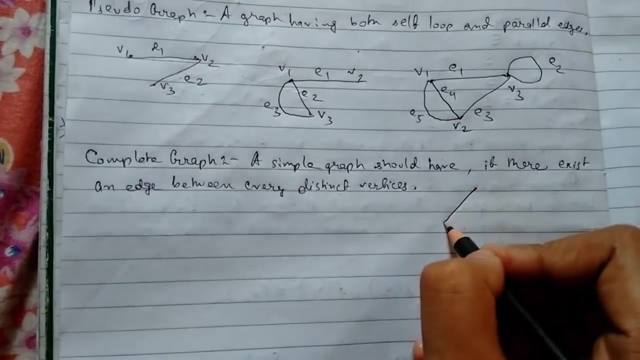 these are parallel edges and this is a simple loop for a complete graph. a simple graph should have this condition: if there exists an edge between every distinct vertices, every distinct edges. so suppose we have something like this: V1, V2, V3, E1, E2, E3. 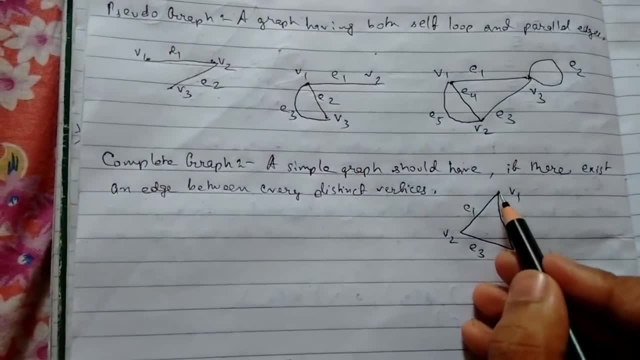 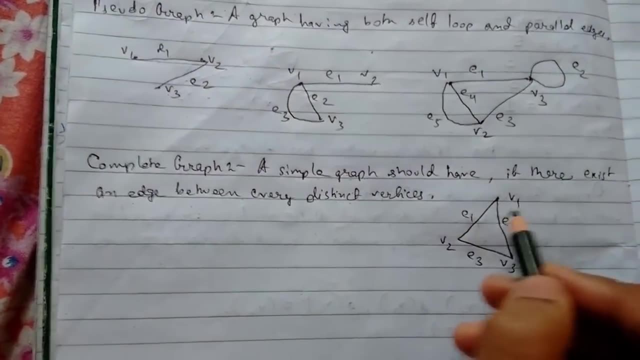 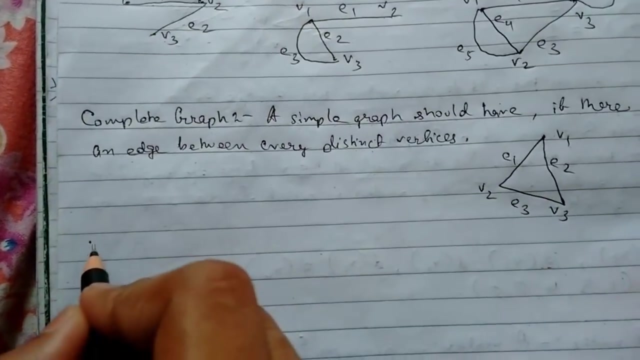 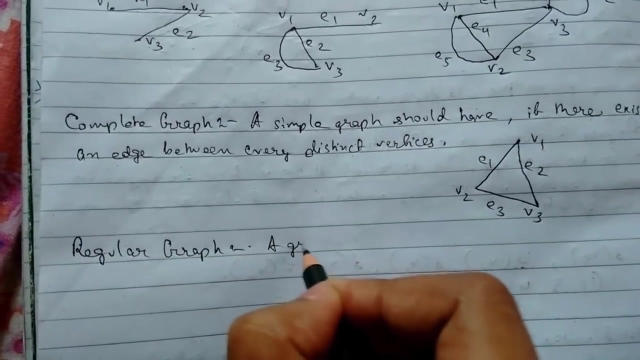 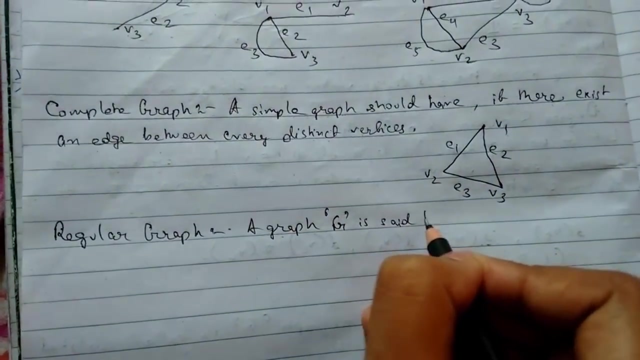 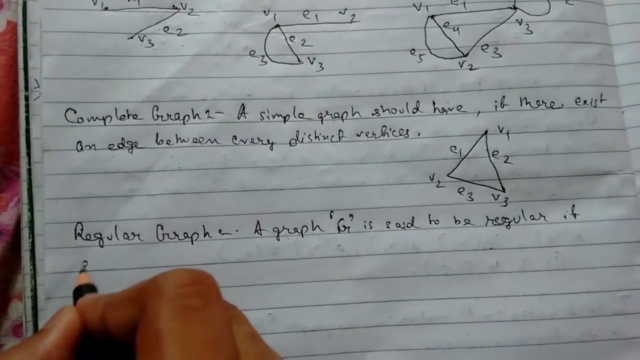 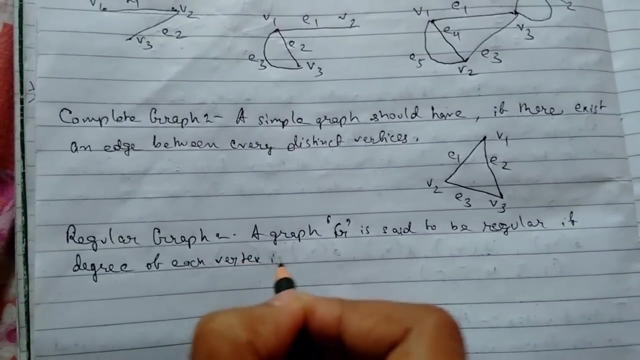 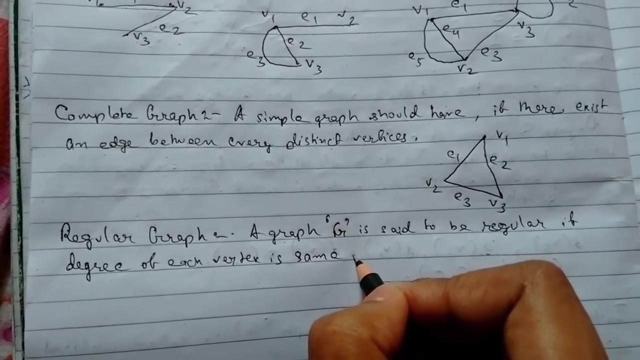 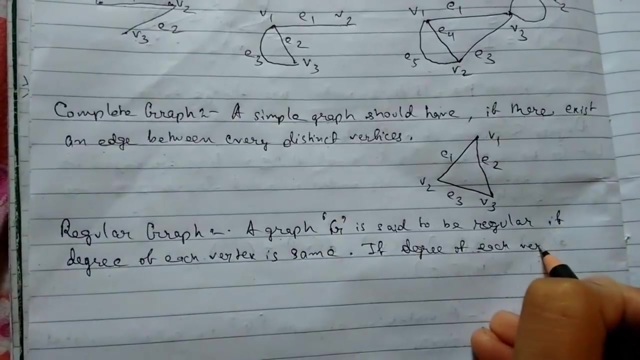 so here we see that each vertex is connected with an edge, so it is continuous. so now let me see regular graph. so a graph G set to be regular if degree of each vertex is same, degree of each vertex is same. so if degree of each vertex is K, 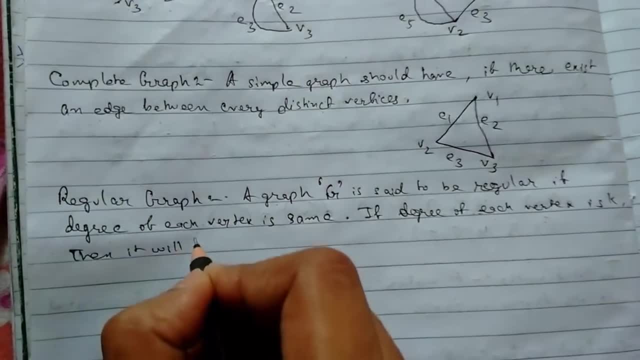 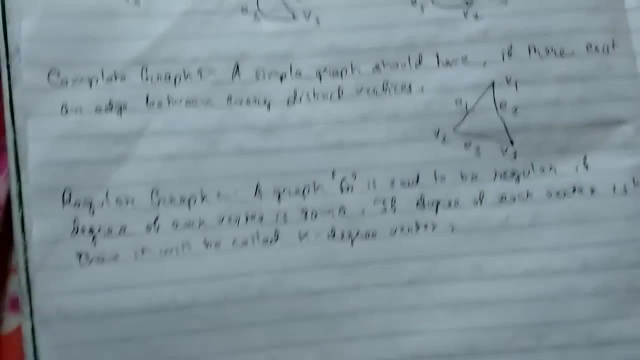 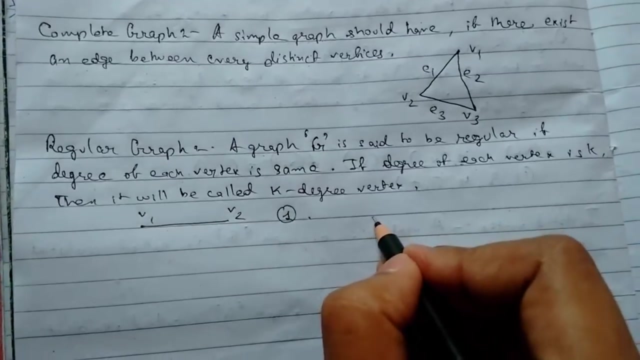 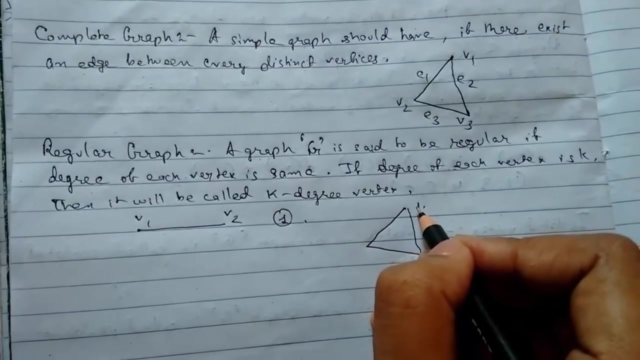 then it will be called K degree vertex. so this for example: suppose V1, V2, so here degree is 1. and for the same example, here we say V1, V2, V3, here is degree 2, 2, 2, so degree 2. 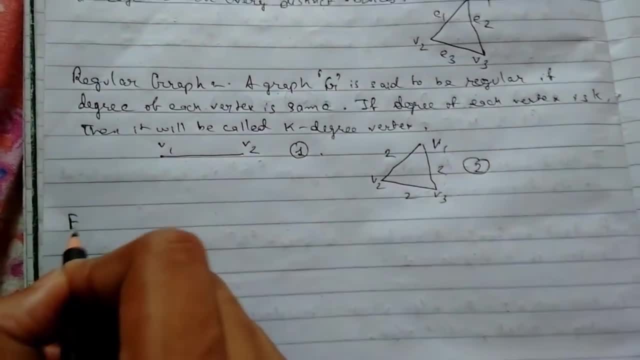 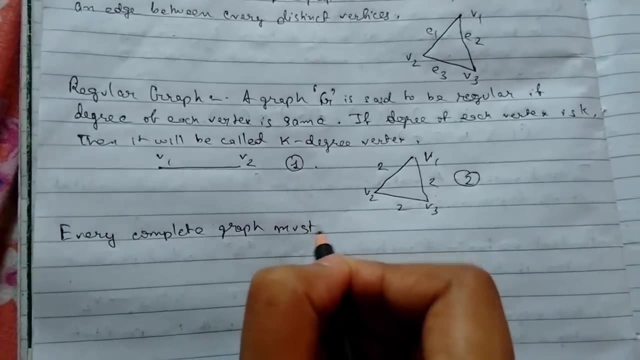 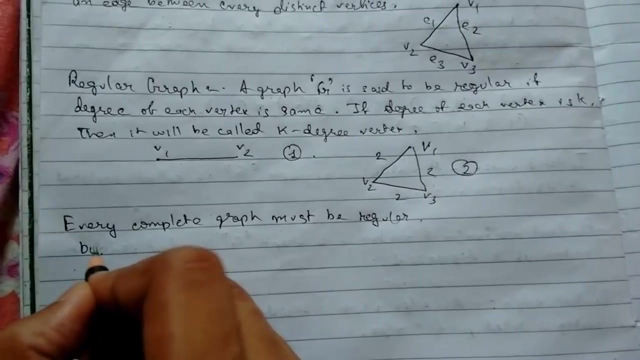 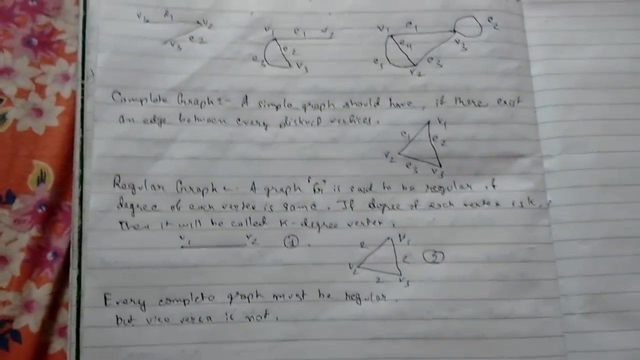 so one important point is that every complete graph must be regular, but vice versa is not same. but vice versa is not, so thank you for watching it. 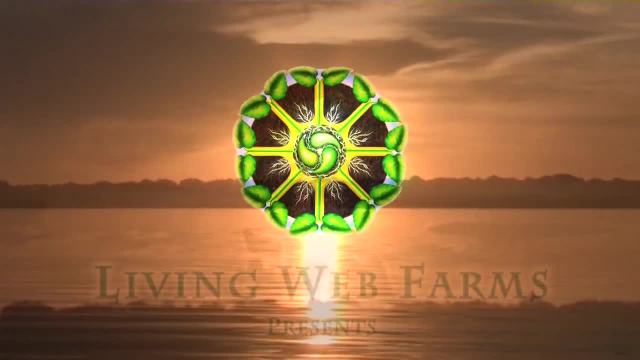 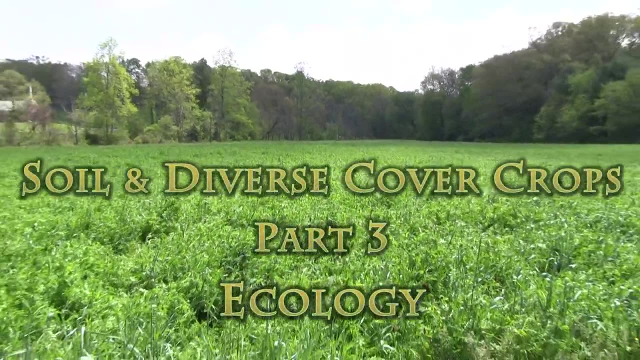 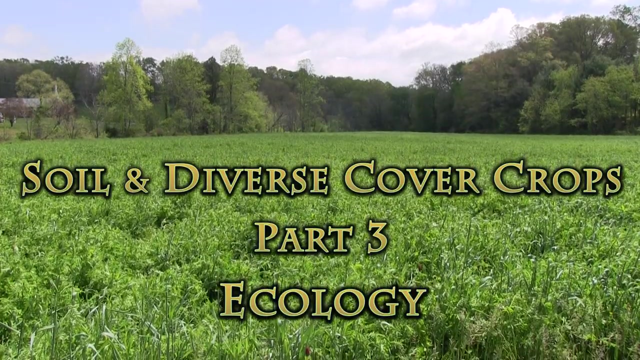 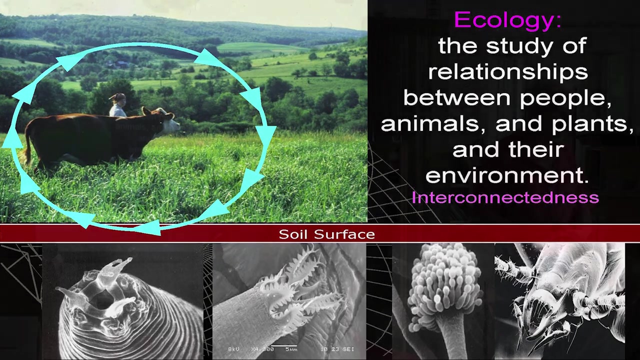 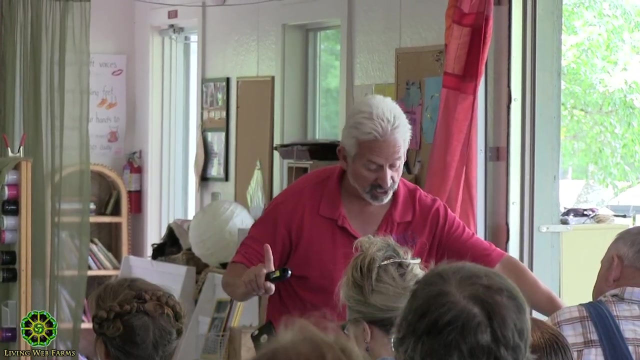 Here's what we're going to do: Connectness- Everything is one, Everything is connected. If you can learn another principle today, everything is connected. So if you do this, what are you doing to this? this, this, this, this, this? I never thought these microbes. 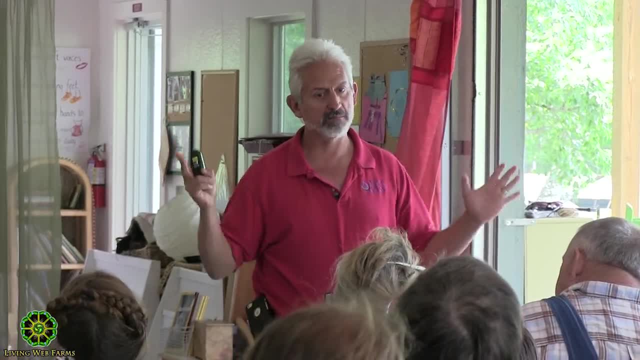 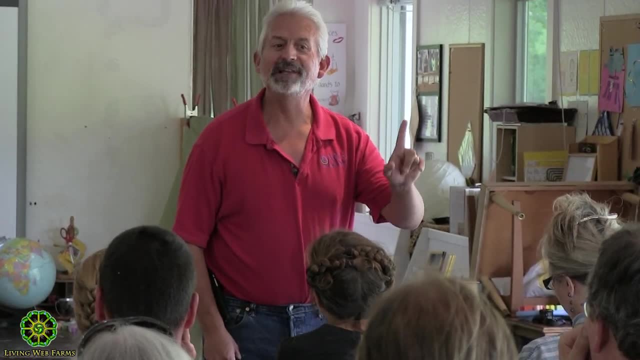 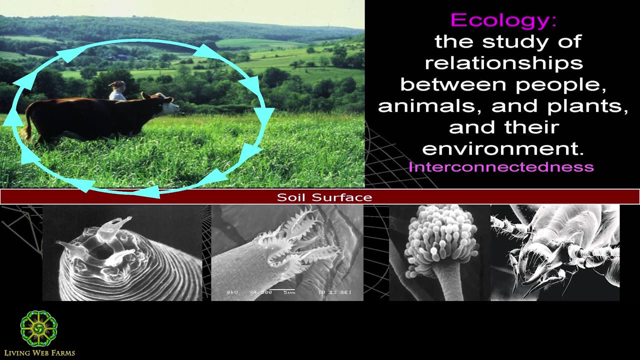 were connected to the water cycle. Who would have thought that microbes are connected to the water cycle? No glues, no infiltration, no completed water cycle. Water cycle is complete when it goes into the soil, not run off and go to the river and lake. That's not a complete. 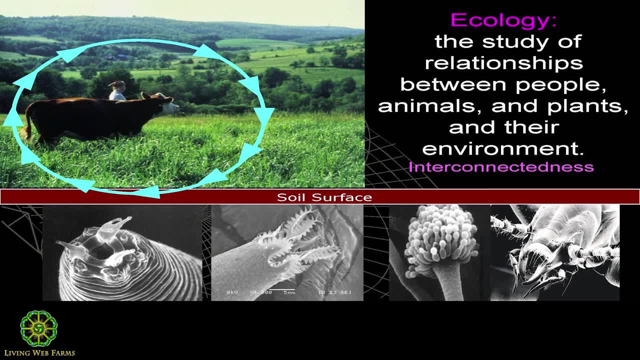 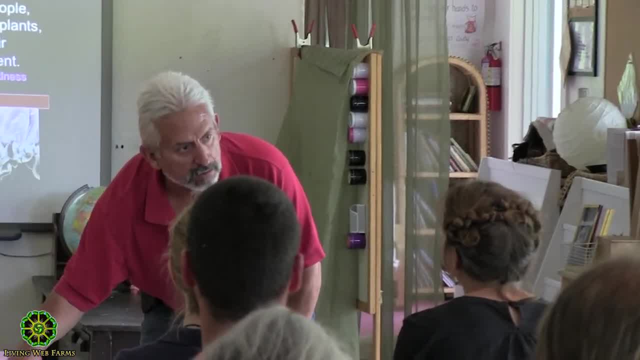 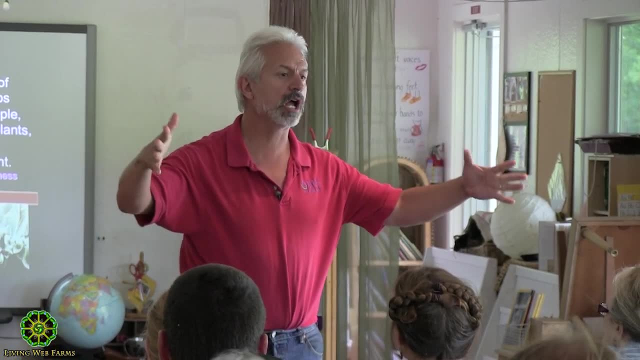 water cycle. Okay, This is proactive farming. You take care of the water the moment it lands on that spot. If it goes to the end of the field on your buffer, game's over, You can put all these nice conservation practices, You can do buffers, You can put terraces, But if you're 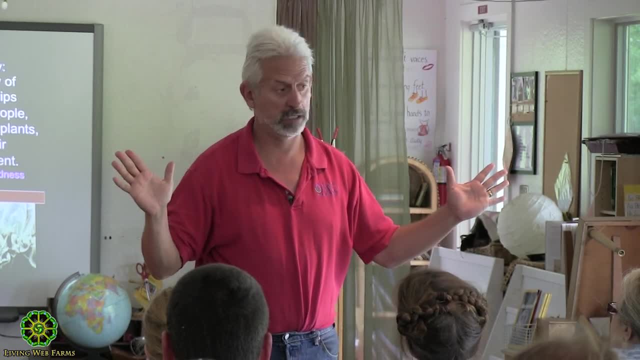 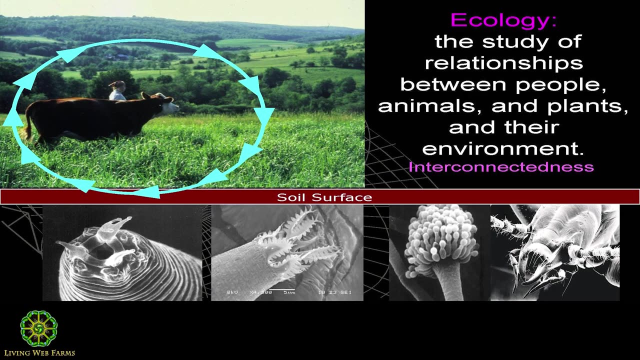 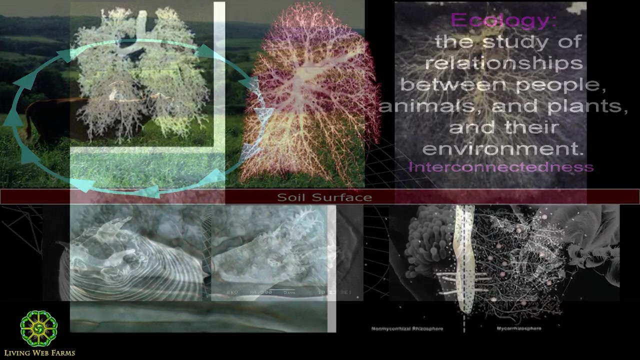 still tilling in between the terraces. we fixed nothing. I got to capture sun energy right here. I got to stop the raindrops. I got to feed and build aggregates right there. Anything else of that is reactive conservation. Nature uses patterns, holes and patterns. This is a human lung Fractals. How many of 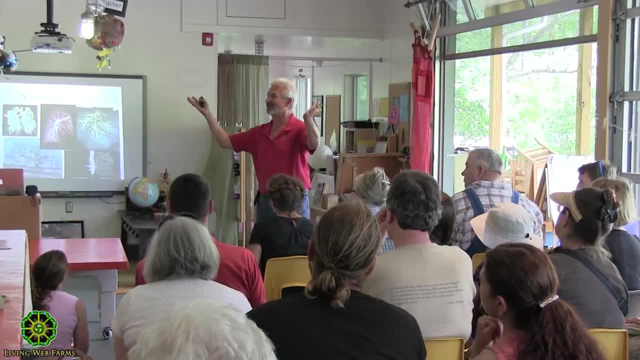 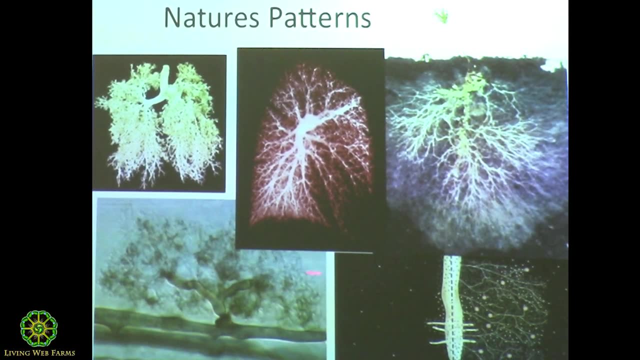 you guys know about fractals. Fractals are cool, aren't they? Mathematical? Yes, Broccoli, mycorrhizal. Look at the patterns. Nature uses patterns. When you see a tree branch out, that's a fractal.